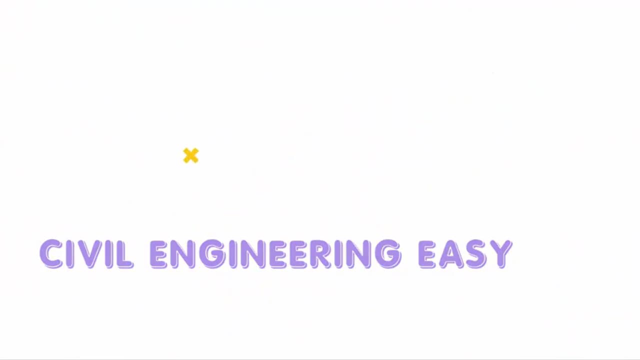 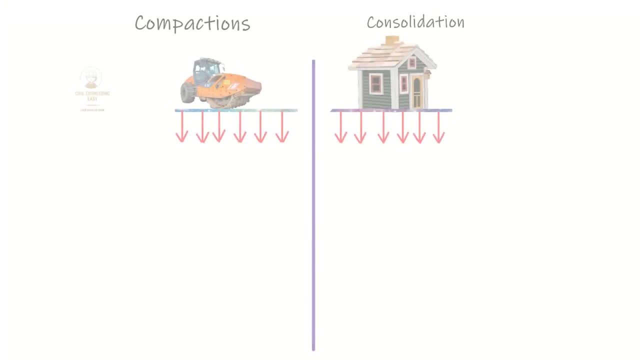 Welcome back. You are watching YouTube channel Civil Engineering Easy. In this short video I will discuss the basic and important topic in soil mechanics, that is, what is the main difference between compaction and consolidation of soil. Following are the difference between compaction and consolidation. First main difference is that the compaction is the compression of soil. 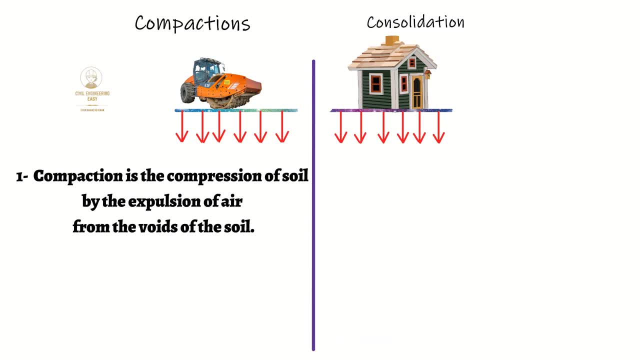 by the expulsions of air from the wires of the soil, While the consolidation is the compression of soil by the expulsions of water from the wires of the soil. The compaction is a quick process, while the consolidation is a slow process. Short-term loading is required for the compaction. 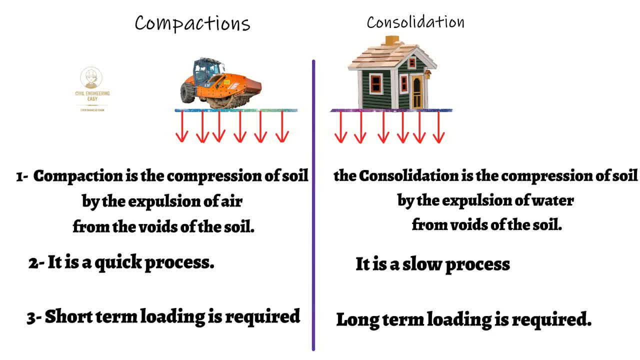 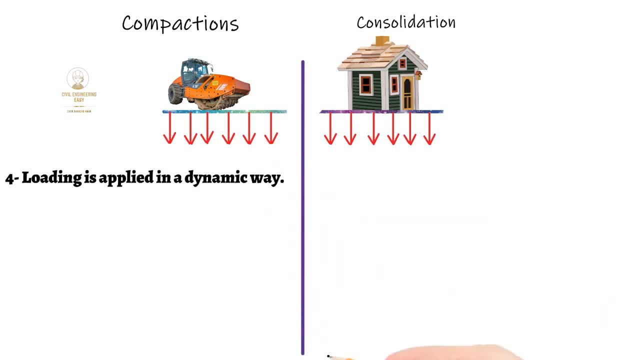 process, while for the consolidation, long-term loading is required. Loading is applied in a dynamic way, that is, compaction with the help of different types of rollers, While in the case of consolidation, loading is static and constant. Any type of soil, either it is cohesion or cohesionless. 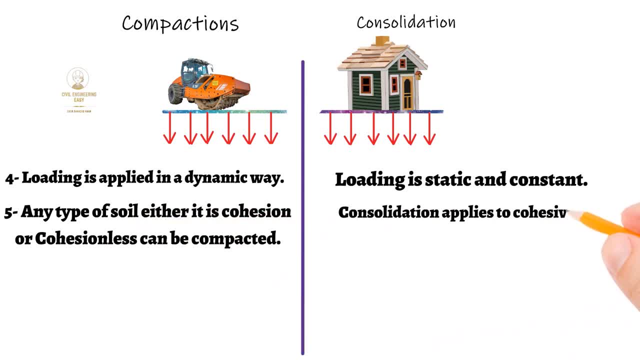 can be compacted, While consolidation applies to cohesive soils only. especially for the low permeable clay, Degree of saturation of soil to be compacted should be less than 100%, While in the case of consolidation, degree of saturation of the soil to be consolidated should be 100%. With the 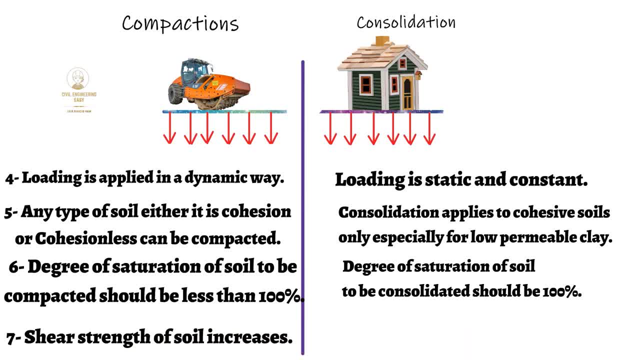 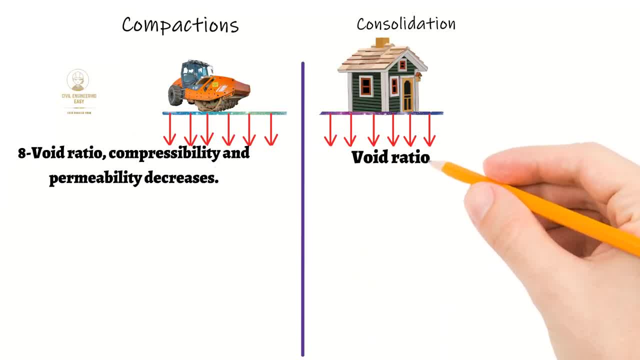 help of compaction, the shear strength of soil increases. In the case of compacted soil, the shear strength of soil increases. Similarly, the shear strength of the soil increases in consolidation. Wired ratio, compressibility and permeability decreases in both compaction and consolidation. 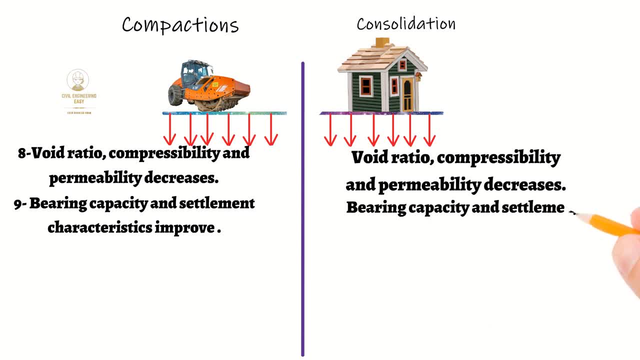 Bearing capacity and settlement characteristics improve in compaction and consolidation. Compaction is done properly in order to get maximum dry density of soil. Compaction is done purposely in order to get the maximum dry density of soil. Consolidation of soil occurs naturally when the structure loads from the foundation. Compaction is done before the construction of a 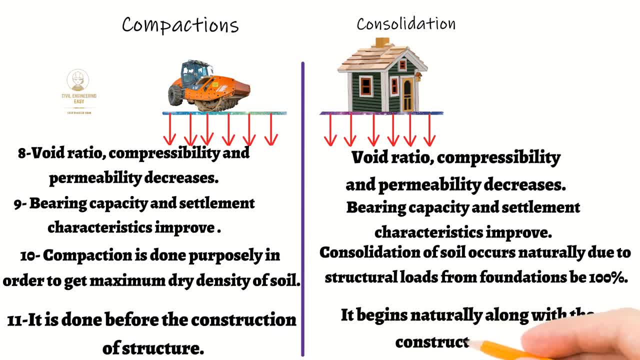 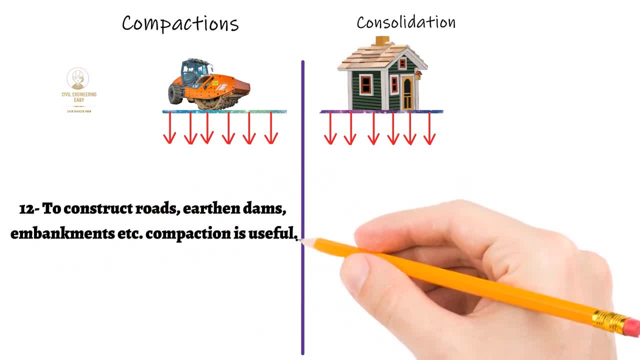 structure, While consolidation begins naturally along with the construction work. To construct roads, earthen dams, embankments, etc. Compaction is useful, While the foundation soil properties will improve over a long period due to consolidation. That's what we discussed.